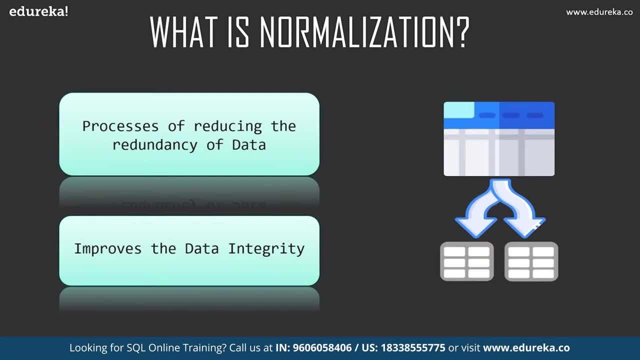 that is present on the database. Well, every table in the database has to be in the normal form. So normalization is used mainly for two purpose. So the first one is it is used to eliminate repeated data. having repeated data on the system not only makes the process slow, 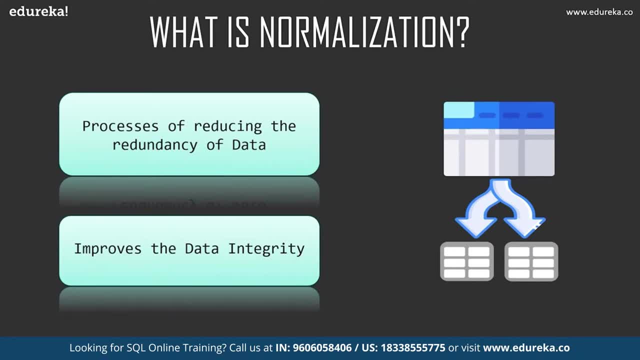 but will cause trouble during the later part of transactions. and second One is to ensure the data dependencies make some logical sense. Yes, usually the data is stored in database with certain logic. huge data sets without any purpose are completely waste. It's like having an abundant resource. 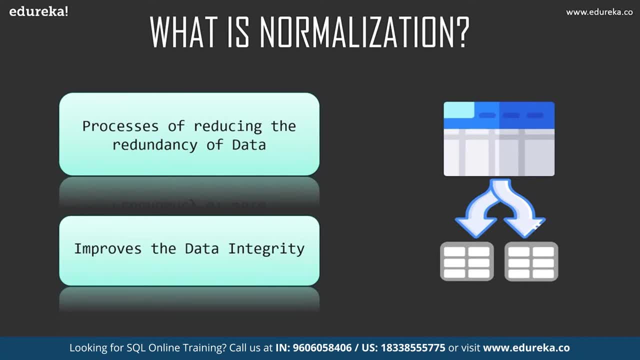 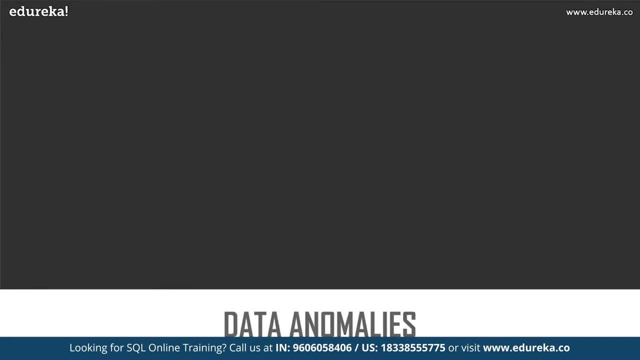 without any application. the data that we have should make some logical sense. normalization came into existence because of the problems that occurred on data. Now let's look at those problems, and these are known as data anomalies: If a table is not proper, only normalized and has data redundancy. 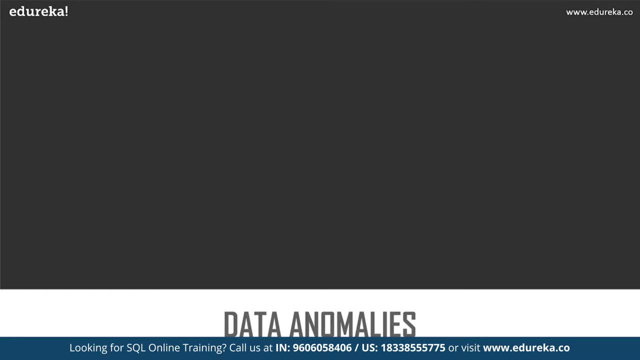 then it will not only eat up the extra memory space but will also make it difficult to handle and update the database. Let's look at the first anomaly, that is, insertion anomaly. Suppose: for a new position in a company, Mr Rakshit is selected. 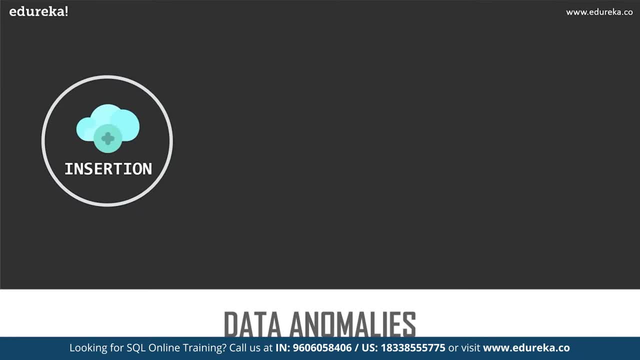 but the department has not been allotted for him. in that case, If we want to update his information to the database, we need to set the department information as null. Similarly, if we have to insert data of thousand employees who are in similar situation, then the department information will be repeated. 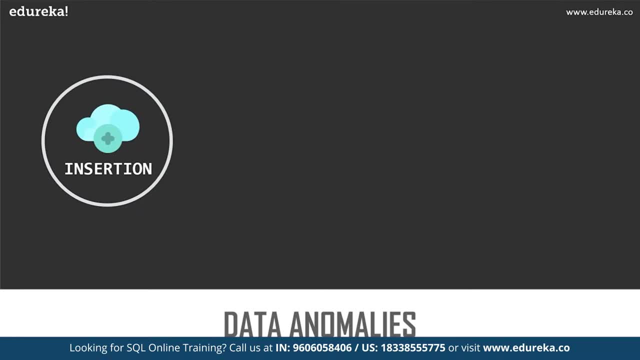 for all those thousand employees. This scenario is a classical example of insertion anomalies. The next one is update anomaly. What if Mr Rakshit leaves the company or is in no longer the head of the marketing department? in that case, all the employee records will have to be updated. 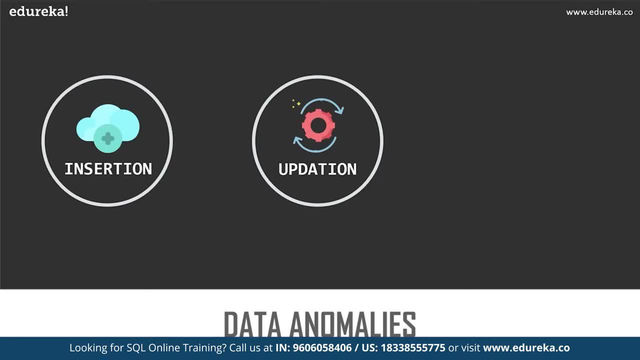 and if, by mistake, we miss any record, it will lead to data inconsistency. This is nothing but updation anomaly. and the final one is deletion anomaly. in our employee table, two different pieces of information are kept together, that is, employee information and department information. Hence, at the end of financial year, 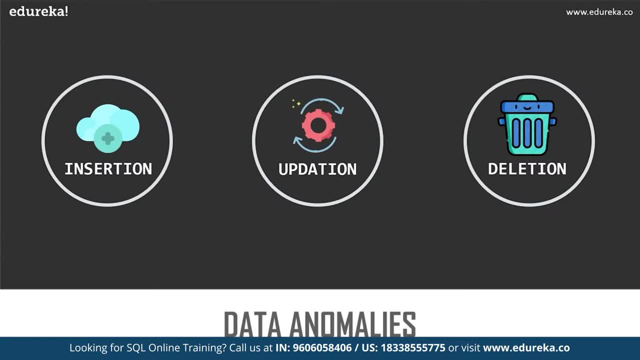 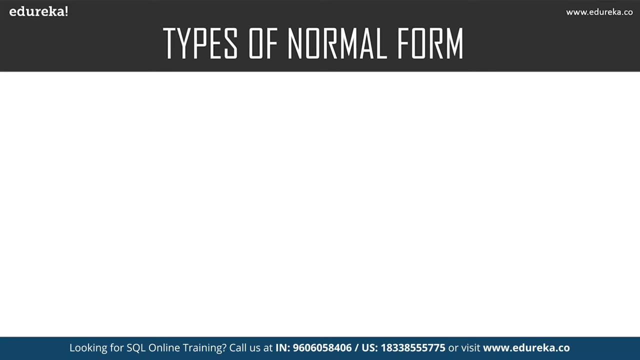 if employee records are deleted, we will also lose the department information. This is nothing but deletion anomaly. So these were some of the problems that occurred while managing the data to eliminate all these anomalies Once normalization came into existence. there are many normal forms which are still under development. 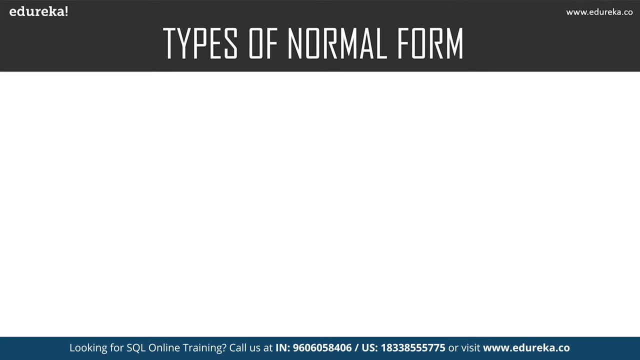 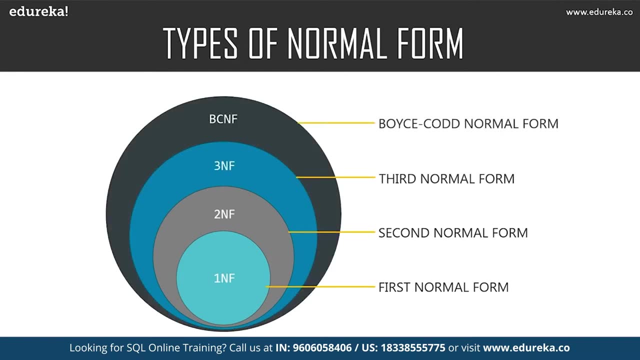 but let's focus on the very basic and the essential ones only. So we will be talking about first normal form, second normal form, third normal form and finally end this session with Boy Scored normal form. So, without wasting further time, let's proceed to first normal form. 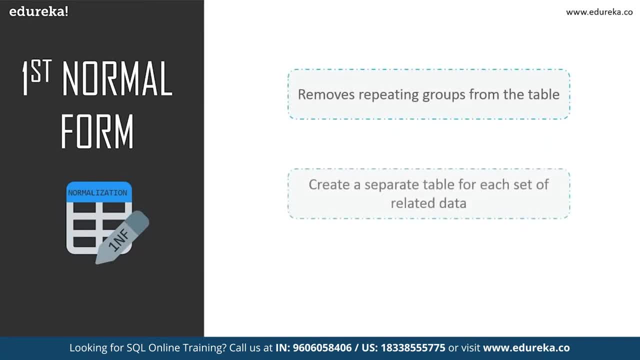 in first normal form. We tackle the problem of atomicity here. atomicity means values in the table should not be further divided. in simple terms, A single cell cannot hold multiple values. If a table contains a composite or multi-valued attributes, it violates the first normal form. 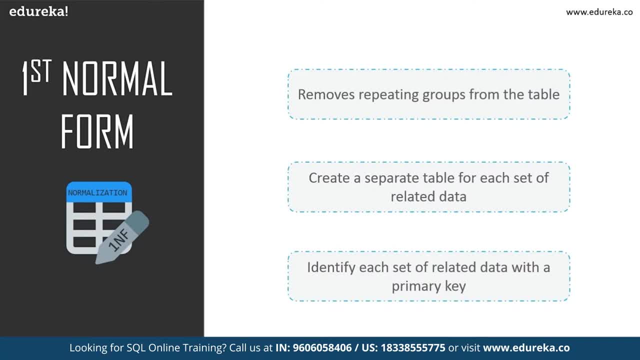 So the following functions will be performed in first, normal form. The first one is it removes repeating groups from the table and next it creates a separate table for each set of related data And finally, it identifies each set of related data with the primary key to understand this in a better way. 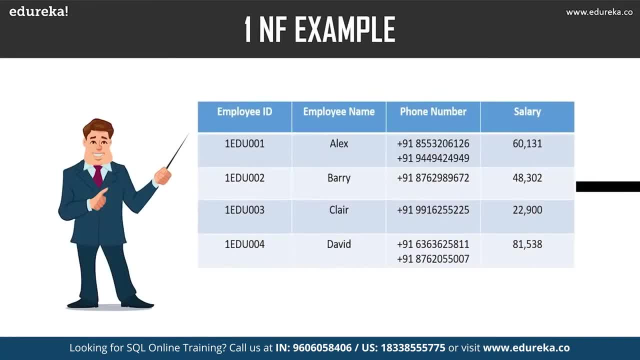 Let's look at the given table. in the employee table We have employee ID, employee name, phone number and salary as columns. We can clearly see that the phone number column has two values. thus it violates the first normal form. Now if we apply the first normal form to the above table, 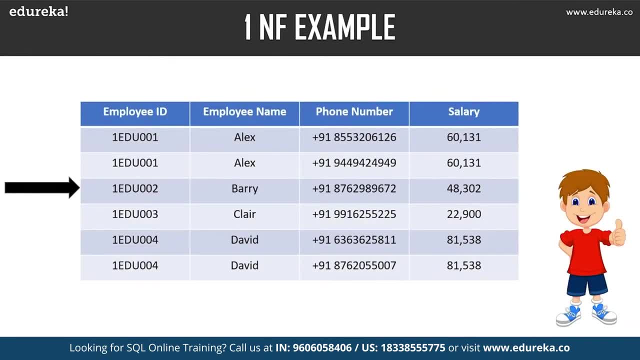 we get the following result: in this table each and every row is distinct, that is, no cell has multiple values. The table has achieved atomicity First. normal form is simple and can be easily identified in the table. We can clearly see there is no multiple values. 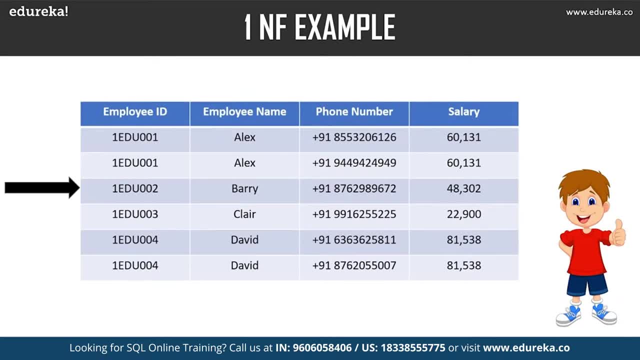 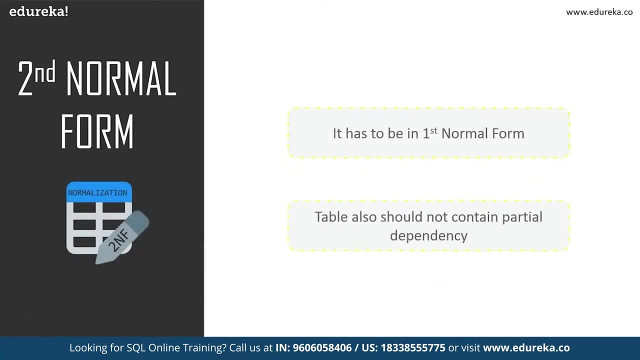 in each and every column. Thus the first normal form is achieved. Now let's move to second normal form. second normal form was originally defined by EF chord in 1971.. A table is said to be in second normal form only when it fulfills the following condition: 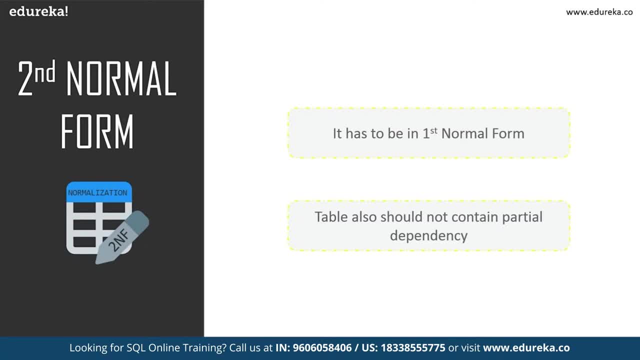 The first condition is it has to be in first normal form, And the second one is the table also should not contain partial dependency. here partial dependency means the proper subset of a candidate key determines a non-prime attribute. So what is a non-prime attribute? 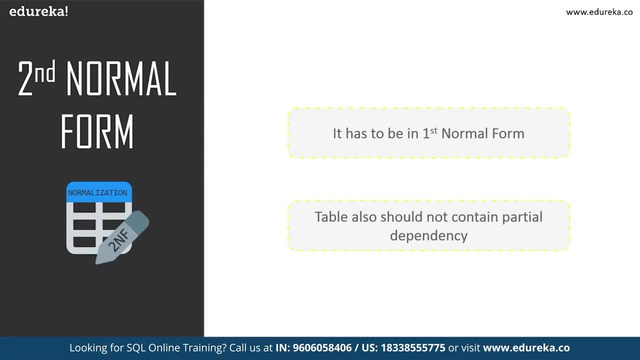 Let's understand this in a simple way. attributes that form a candidate key in a table are called prime attributes and the rest of the attributes of the relation are non-prime. for a table, prime attributes can be like employee ID and Department ID and the non-prime 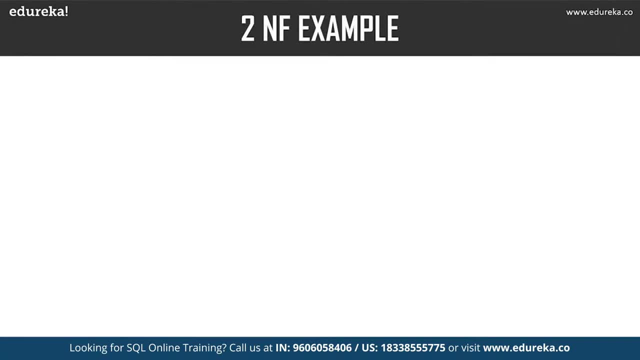 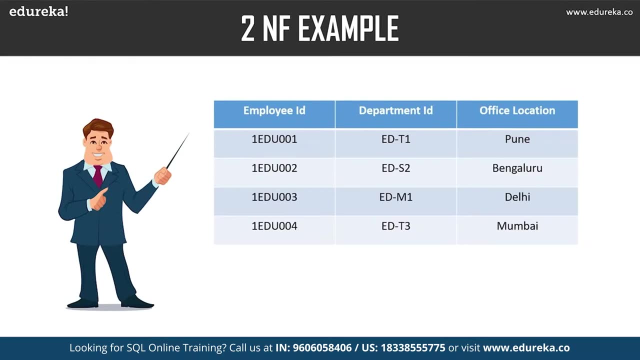 Attributes can be like office location. to understand second normal form, Let's consider this table. This table has a composite primary key that is employee ID and Department ID makes the primary key The non-key attribute is office location. in this case, office location only depends on Department ID. 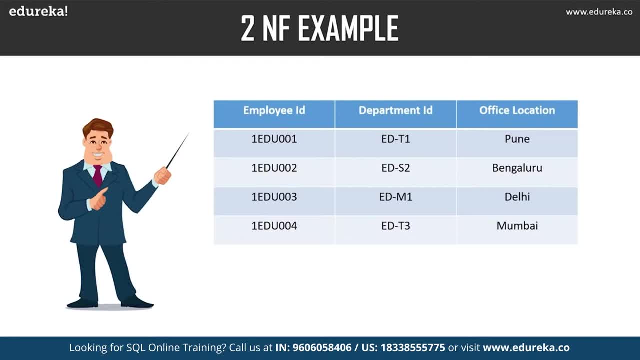 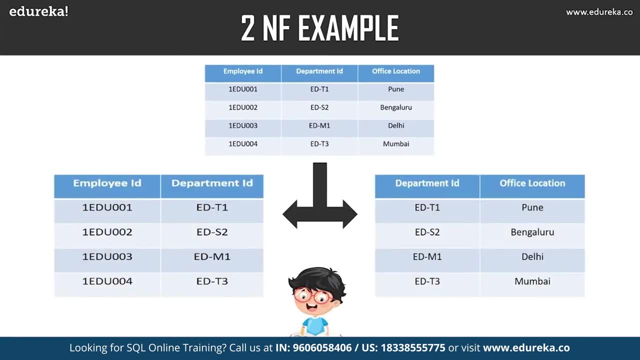 which is only the part of primary key. Therefore, this table does not satisfy the second normal form. So what to do in such scenario? The answer is simple: split the table accordingly. to bring this table to second normal form, We need to break the table into two parts. 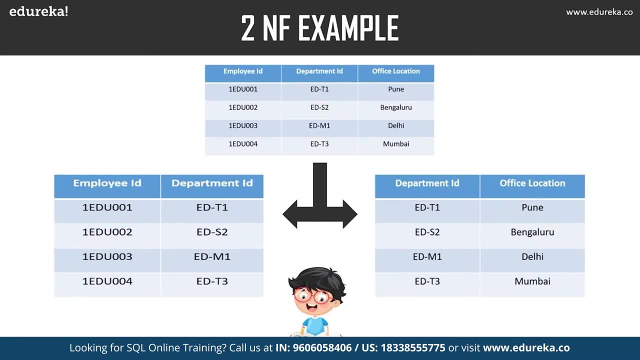 which will give the following tables. The first table has employee ID and Department ID as columns. The second one has Department ID and office location as columns. as you can see, we have removed the partial functional dependency that we initially had. now in the table, The column office location is fully dependent on the primary key. 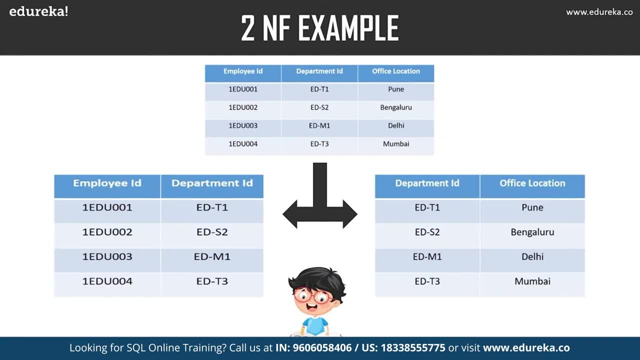 of that table, which is nothing but Department ID. I hope you have understood second normal form. Now that we have learned first normal form and second normal form, Let's head to the next part of this normalization. Next topic is third normal form. 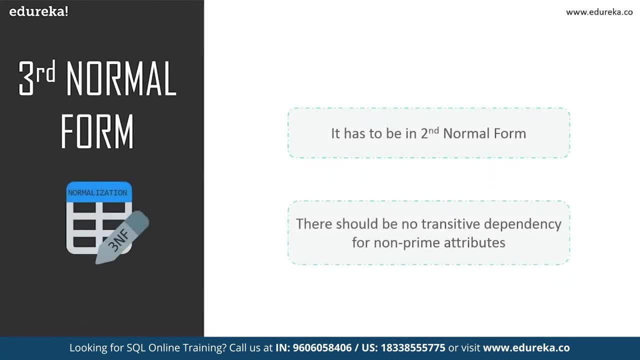 Third normal form is a normal form that is used in normalizing the table to reduce the duplication of data and ensure referential Integrity. The following condition has to be met by the table to be in third normal form, And the first condition is the table. 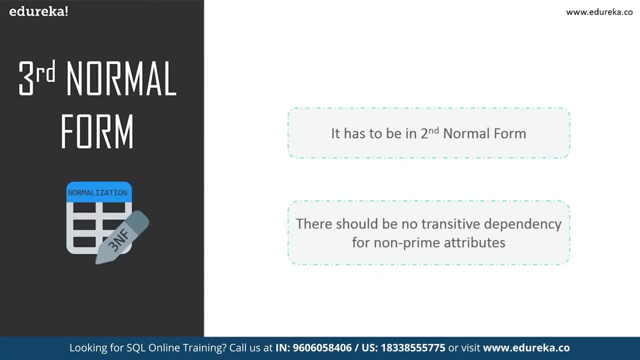 The table has to be in second normal form and the second condition is: no non-prime attribute is transitively dependent on any non-prime attribute which depends on other non-prime attributes. I know it's a bit confusing, So let me make it simple for you. 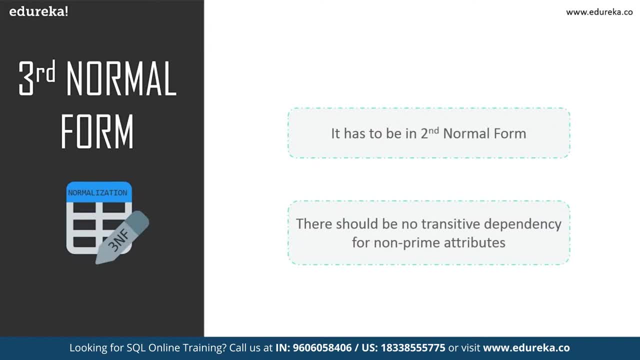 It's like if C is dependent on B and in turn B is dependent on a, then transitively C is dependent on a. this should not happen. in third normal form, all the non-prime attributes must depend only on the prime attribute. So these are the two necessary condition. 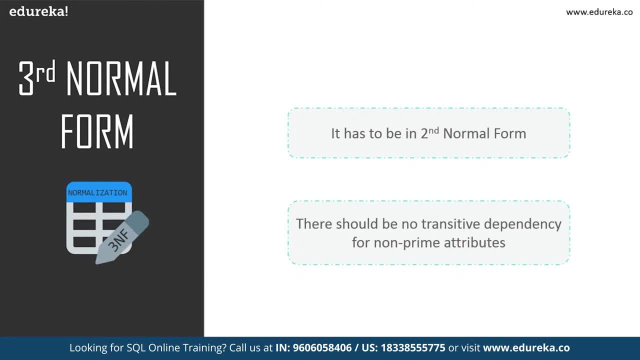 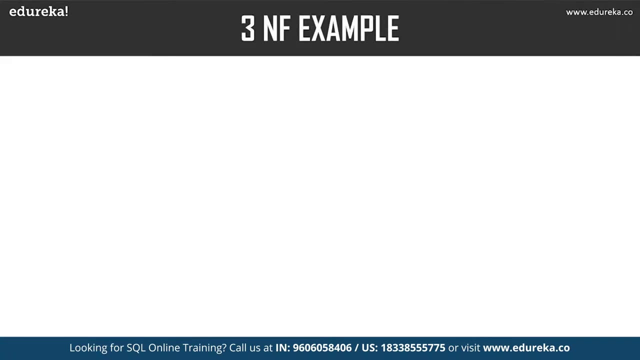 that needs to be attained. So why was the normal form designed? firstly, to eliminate undesirable data anomalies. Next one is to reduce the need for restructuring over time. Finally, to make the data model more informative. since we have understood the third normal form, Let's look at the example table. in the above table, student ID. 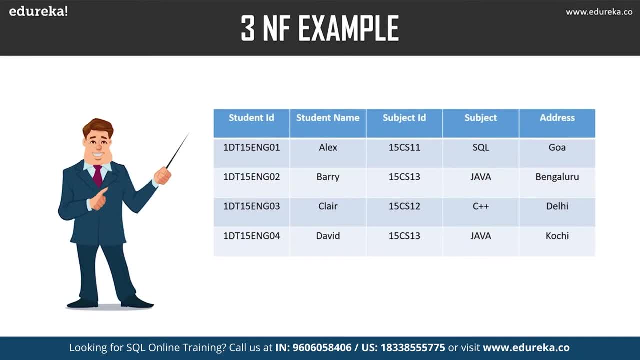 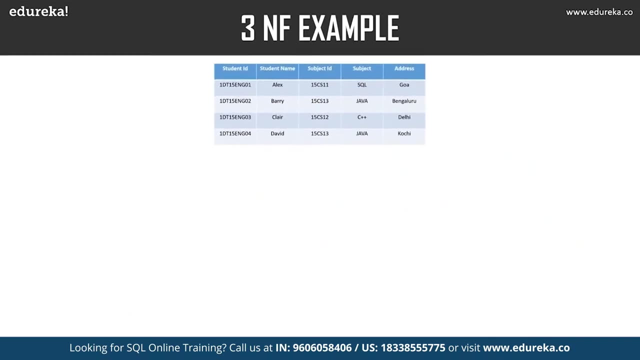 determines subject ID and subject ID determines subject. therefore, student ID determines subject via subject ID. This implies that we have transitive functional dependency and this table does not satisfy the third normal form. now, in order to achieve third normal form, We need to divide the table as shown below. 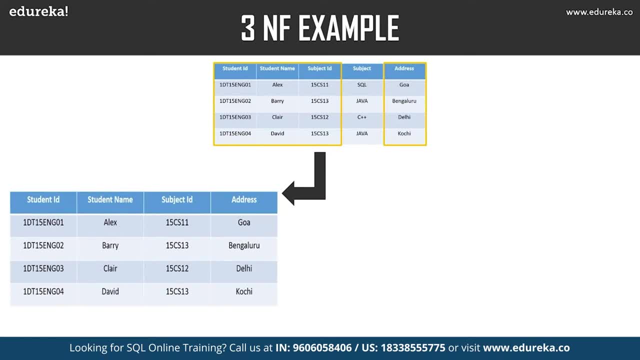 Firstly, let's divide the table and store student ID, student name, subject ID and address in it. All the columns are referring to the primary key, which is student ID. Let the second table have subject ID and subject column. So subject is dependent only on subject ID. 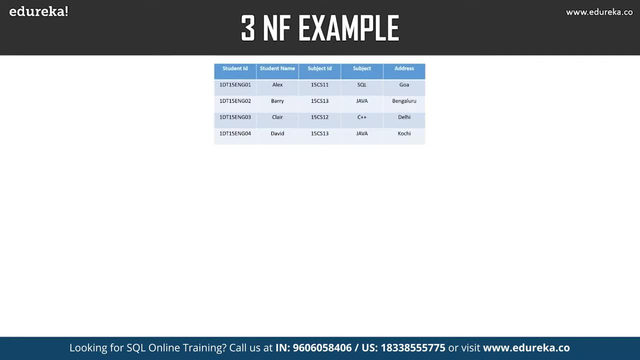 and not on student ID. as you can see from the above table, All the non-key attributes are now fully functionally dependent only on the primary key. in the first table, columns such as student name, subject ID and address are only dependent on student ID. in the second table, subject is only dependent on subject ID. 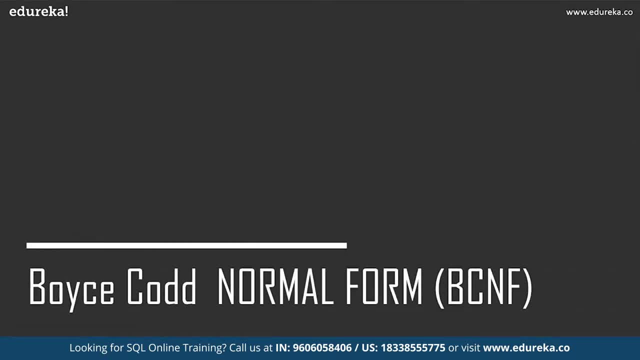 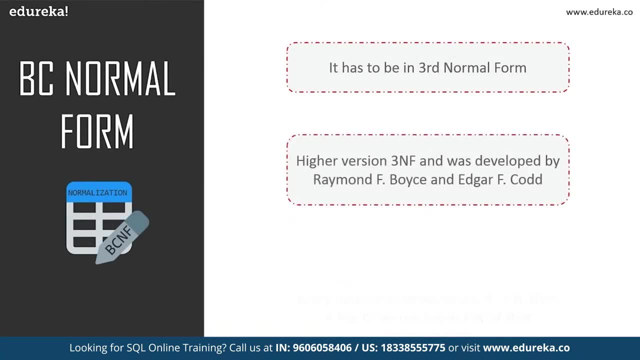 with this being understood Now we can proceed further to next normal form, That is, Boyce-Cord normal form. This is also known as 3.5 normal form. It is the higher version of third normal form and was developed by Raymond F. 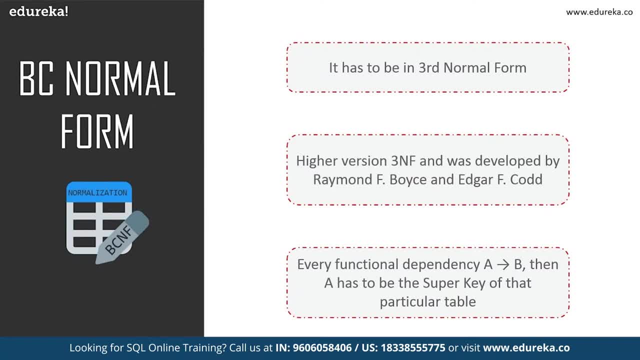 Boyce and Edgar F Cod to address certain types of anomalies which were not dealt with. third normal form: before proceeding to Boyce-Cord normal form, The table has to satisfy: third normal form in Boyce-Cord normal form If every functional dependency, that is, a, implies B. 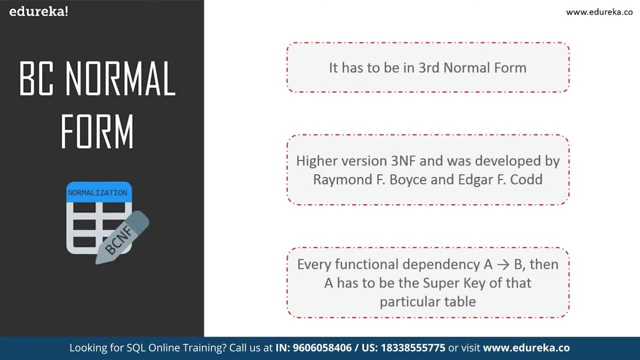 then a has to be the super key of that particular table. So what is a super key? A super key is a group of single or multiple keys which identifies rows in a table. Let's look at the table to clearly understand. Boyce-Cord normal form. 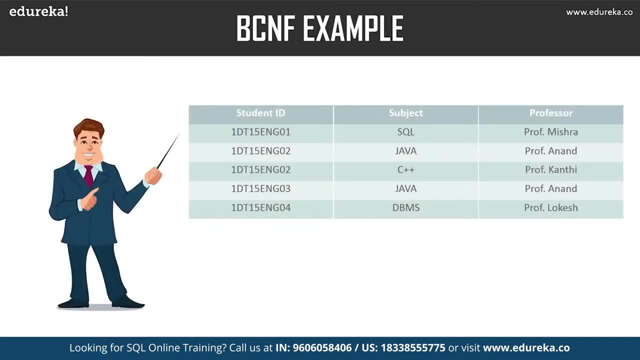 in the given table One student can enroll for multiple subjects. There can be multiple professor teaching one subject and for each subject a professor is assigned to the student. These are the necessary condition of this table. in this table all the normal forms are satisfied except Boyce-Cord normal form. 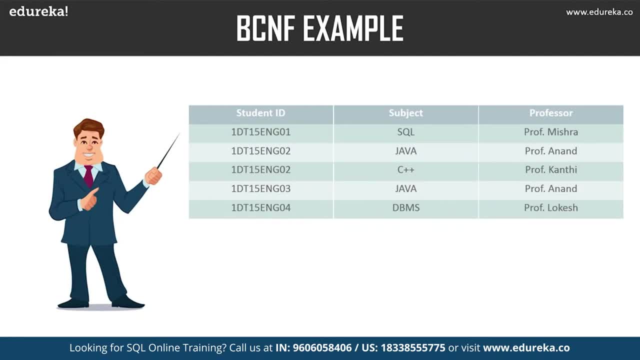 Why, as you can see, that student ID and subject form the primary key, which means that the subject column is prime attribute. but there is one more dependency, that is, professor is depending on subject, and while subject is a prime attribute, professor is a non-prime attribute. 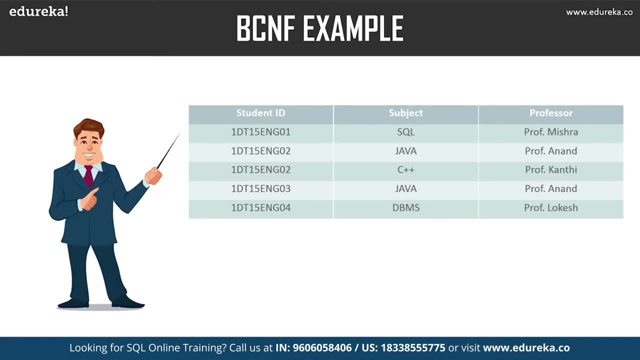 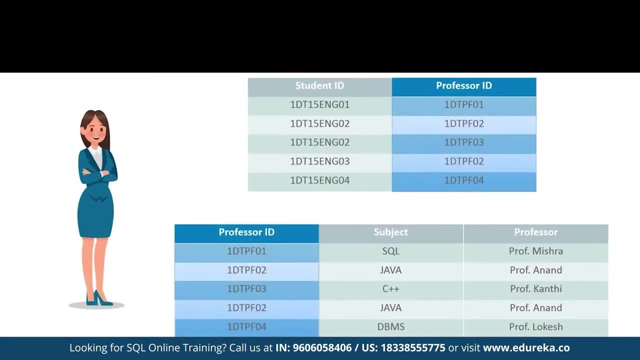 which is not allowed by Boyce-Cord normal form. Now, in order to satisfy the Boyce-Cord normal form, We will be dividing the table into two parts. the table at the top will hold student ID, which already exists, and we will create a new column that is professor ID. 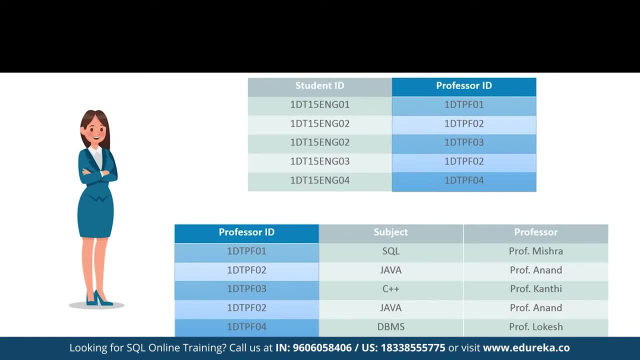 and in the second table, which is below, will have the columns professor ID, professor and subject columns. Why do we need to have a new column, that is professor ID? by doing this We are removing the non-prime attributes- functional dependency. in the second table, professor ID will be the super key. 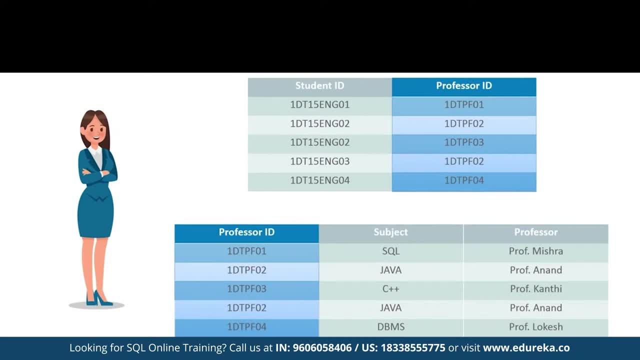 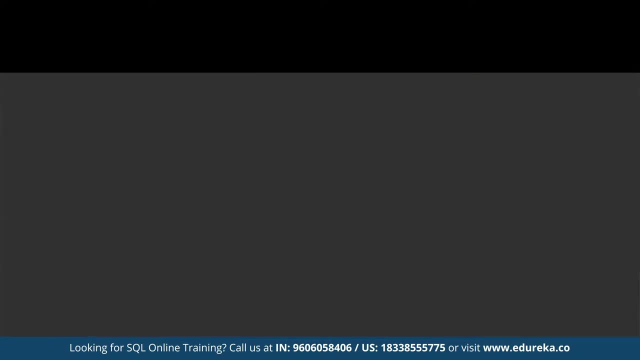 of that table and remaining column will be functionally dependent on it. by doing this, We are satisfying Boyce-Cord normal form. So this brings us to the end of this session. I hope you have clearly understood the normalization and it's different types.